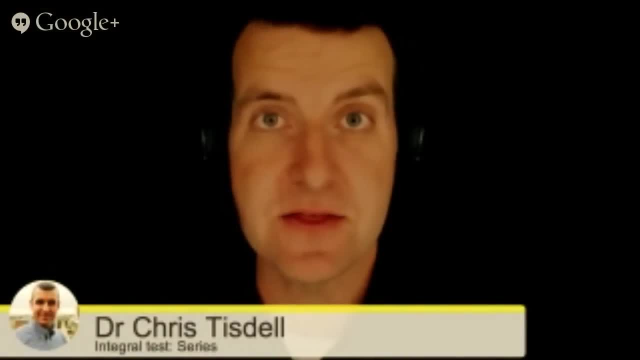 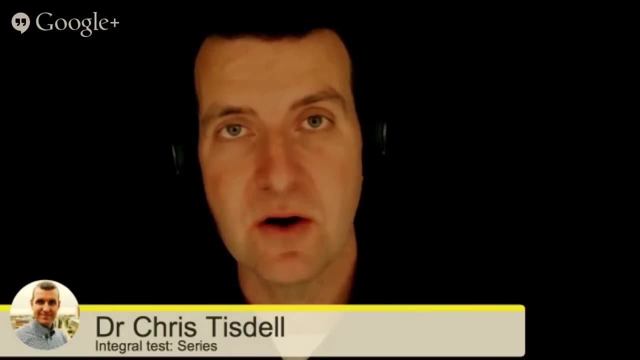 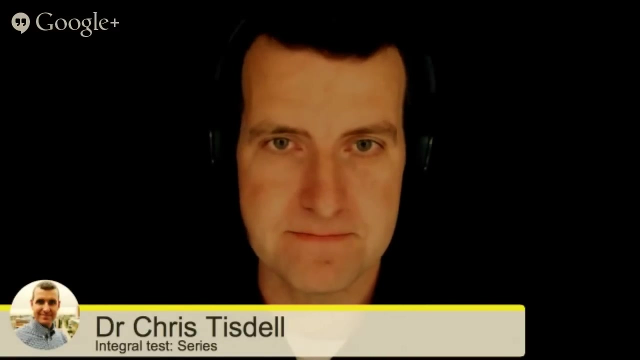 have heard of series in other contexts, for example Fourier series, power series, Taylor series. All these sorts of series pop up in applied mathematics but as a basic starting point these are just series of positive and constant terms, So we also have to do something about the number of some type. 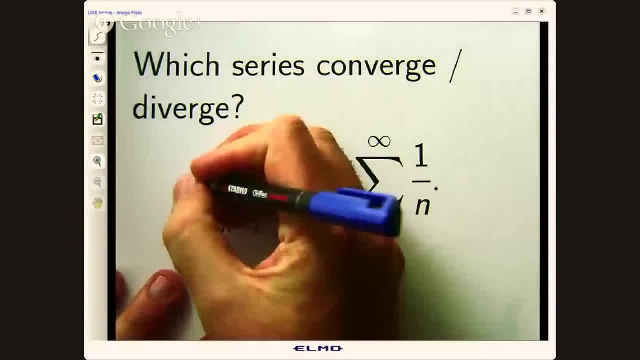 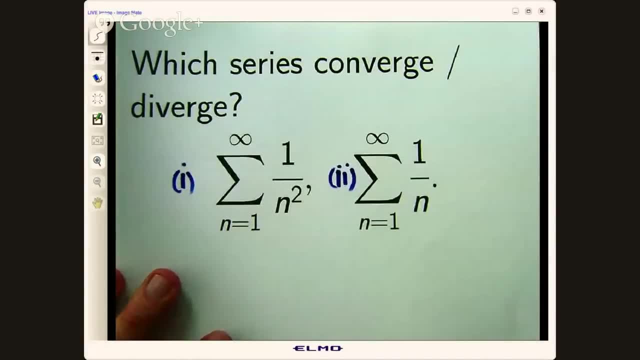 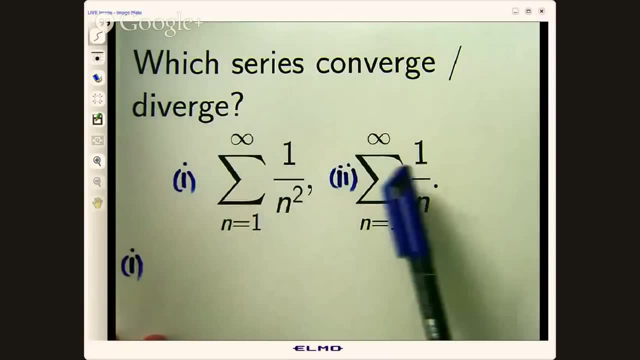 All right, so I'm going to show you this integral test, So let's call this one and this two if you like, and we're going to work through each of these examples. Okay, so now both of these series are known as P series. So you have this one on n to some power. Here the power is two and here the 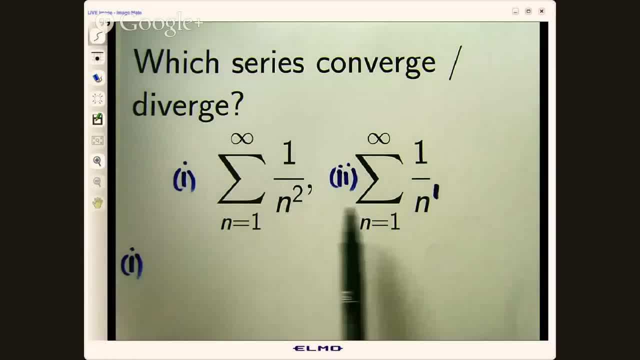 power is one. So you've got one on n to some power, and here the power is two. So you've got one on n to some power, and here the power is two. Now, the value of this power, p tells you whether or not these series converge or diverge. 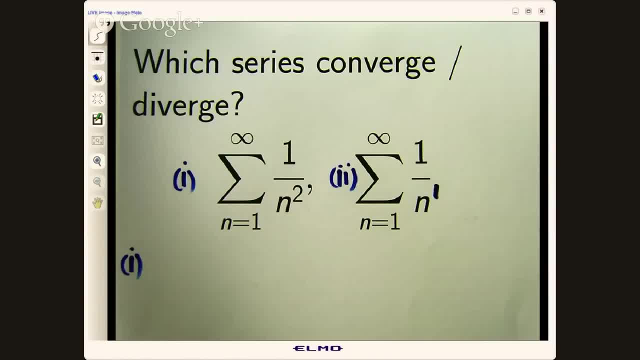 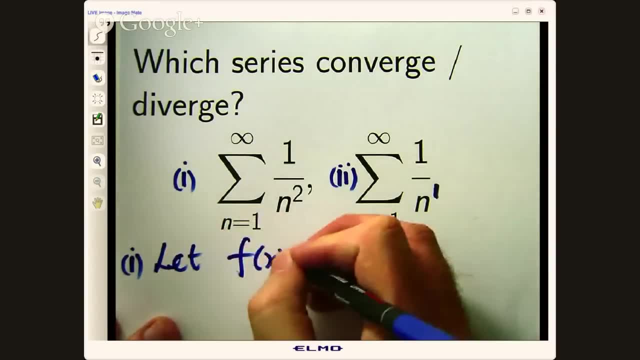 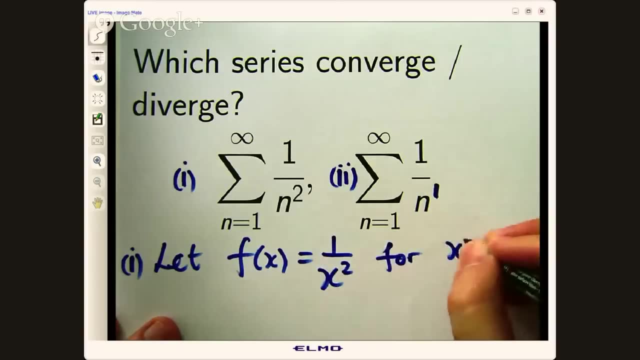 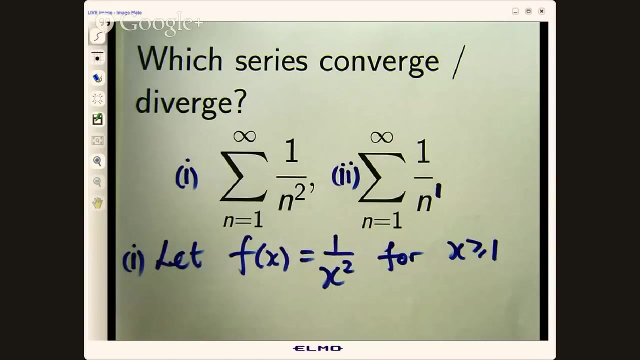 as we'll see from this so-called integral test. Okay, so, for part one, what I'm going to do is I'm going to let f of x be a function associated with the sum, and, Okay, so I've introduced this function of x, x squared, where x is real and greater than or equal to 1.. 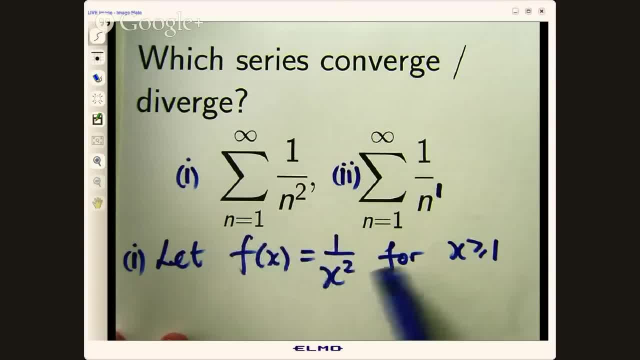 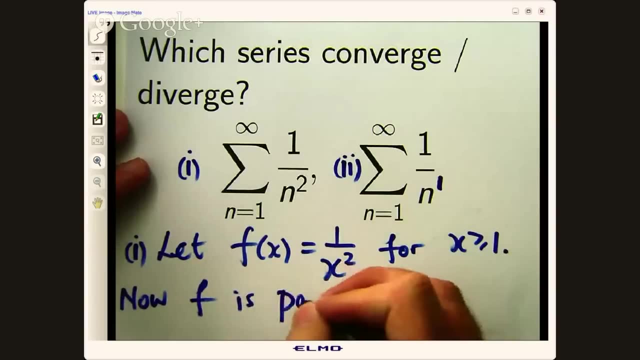 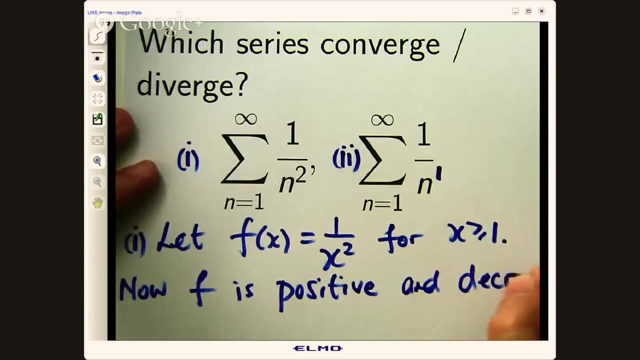 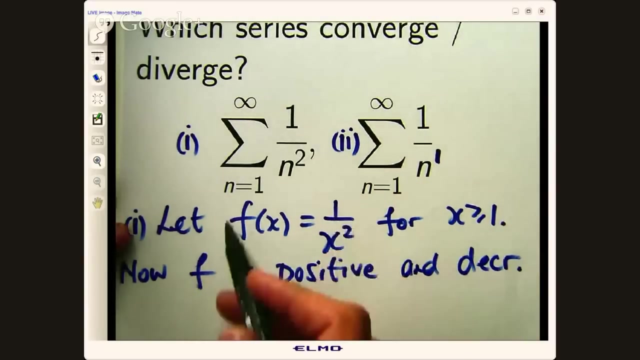 Now, this function is positive for x greater than or equal to 1, and it's decreasing. Okay, these are the two conditions of this integral test: It's positive And decreasing. So what we're going to do now is look at the improper integral of this over the interval from 1 off to positive infinity. 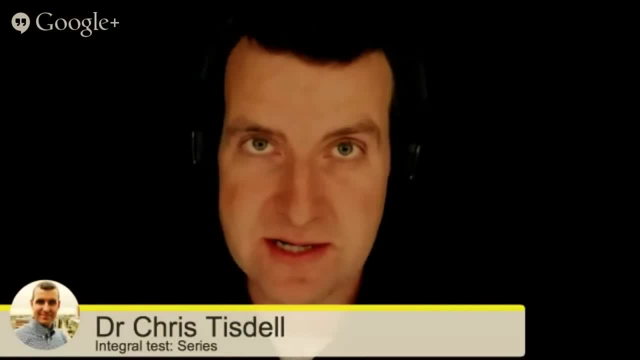 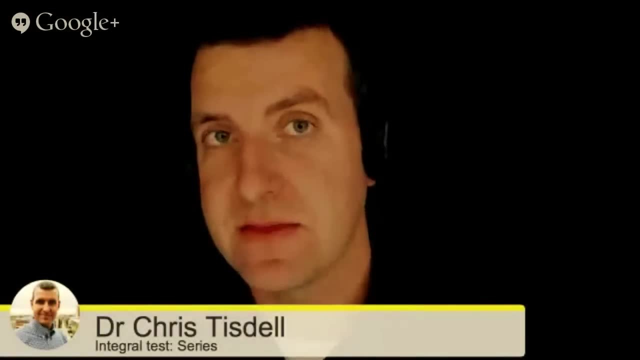 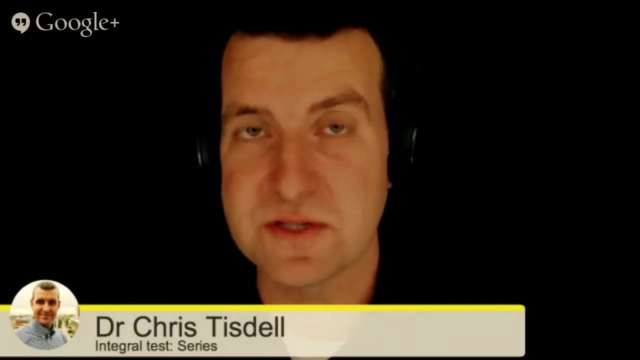 So now this is where the integration comes in in the integral test. If the integral, the improper integral that we're going to calculate, if it converges, then the series also converges. If the integral diverges, then the series also diverges. 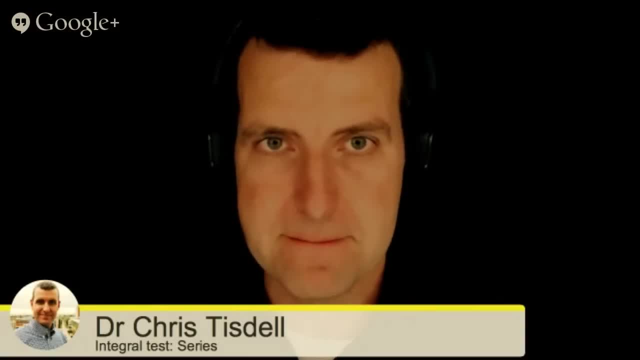 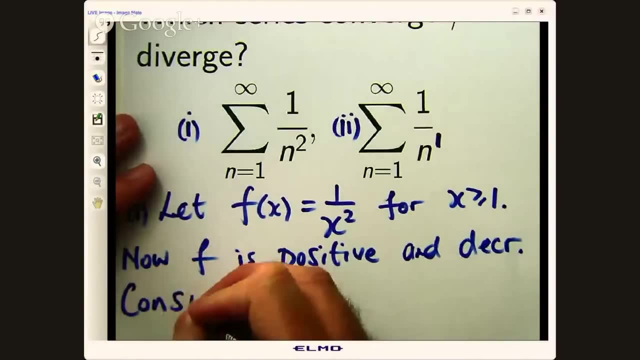 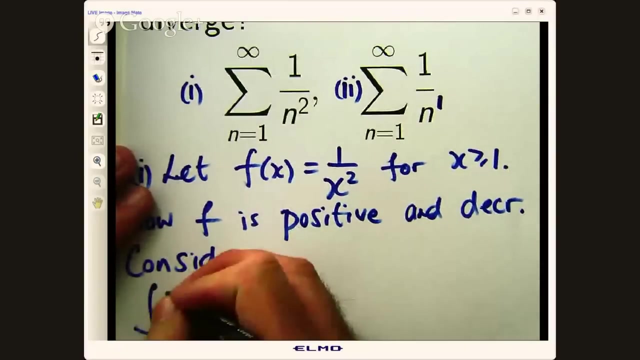 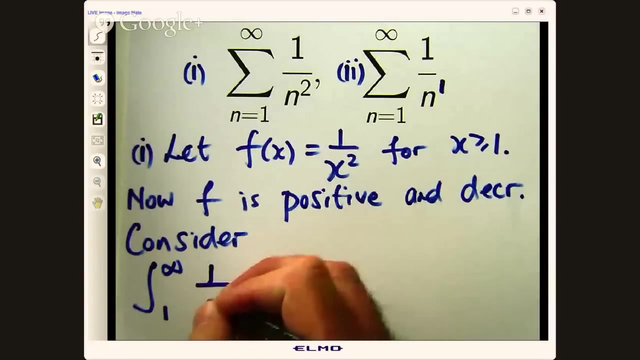 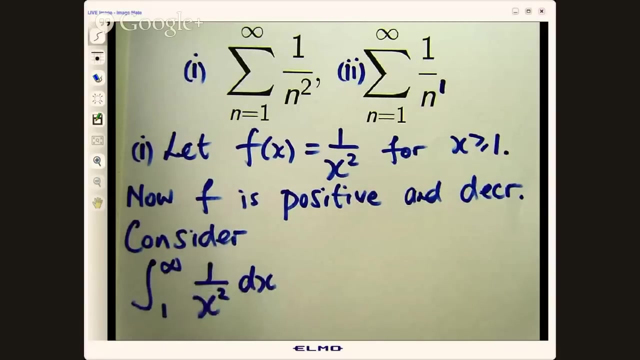 So let me show you what I mean. Okay, so consider the following integral: So I'm going to integrate from x equals 1 off to Positive infinity. So I'm going to have this improper integral. And now you learn about these improper integrals in, say, a first course in calculus or a first course in university calculus. 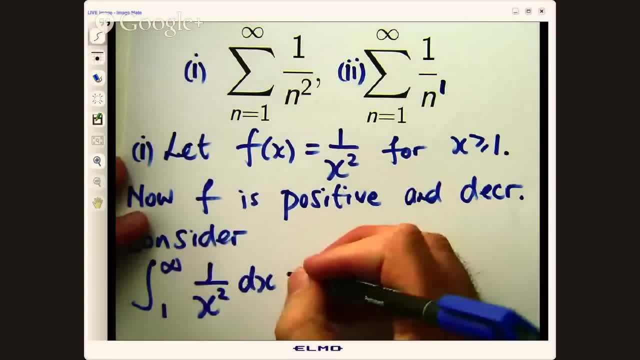 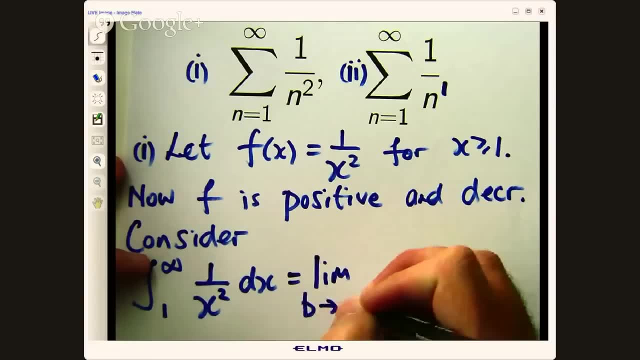 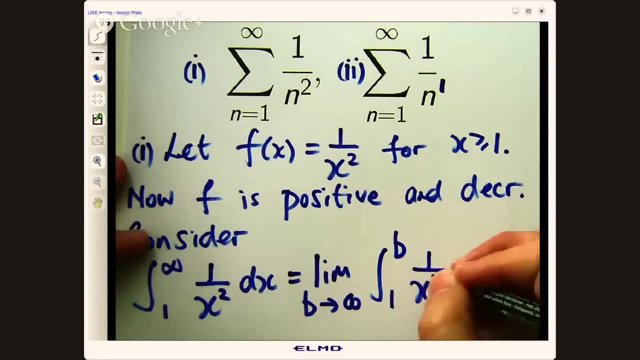 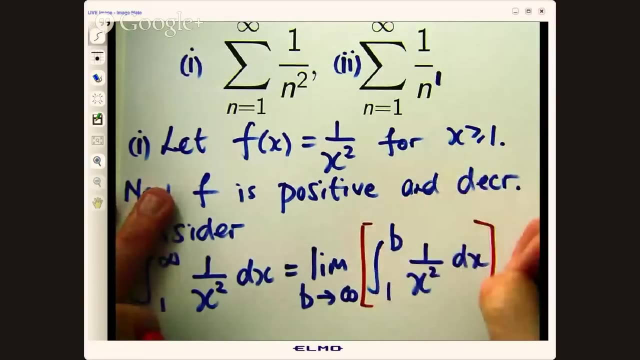 Okay, so you can write this a few different ways. Firstly, you can replace the infinity with a limit, And So B, And what you do is you do this integration first and then you'll take the limit. Okay, so let's do that. 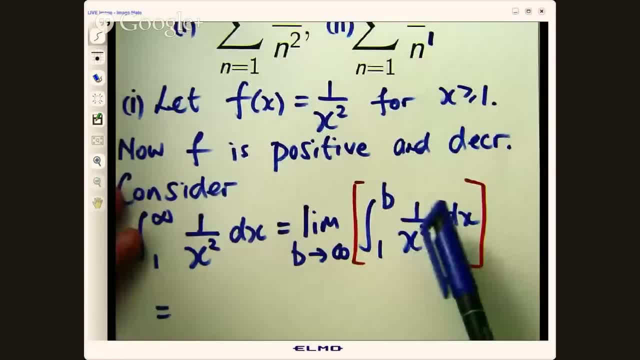 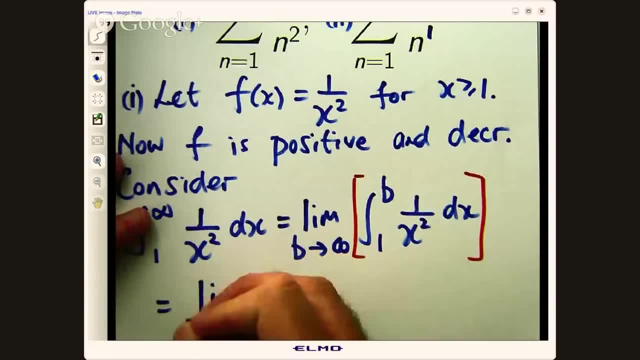 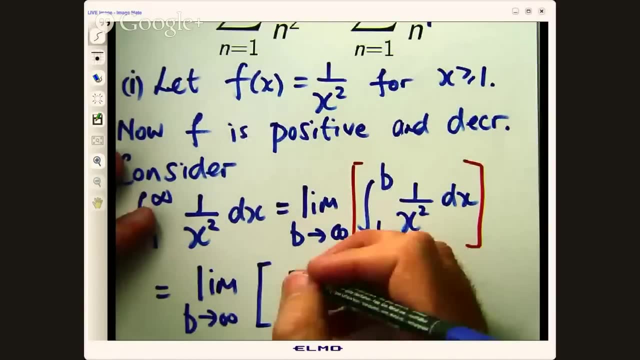 So if I integrate this, it's like x to the minus 2.. I increase the power by 1 and I divide by the new power. So it's going to be something like this. So it's going to be something like negative 1 on x. 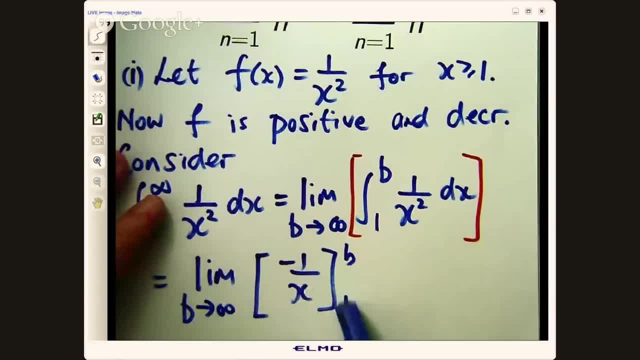 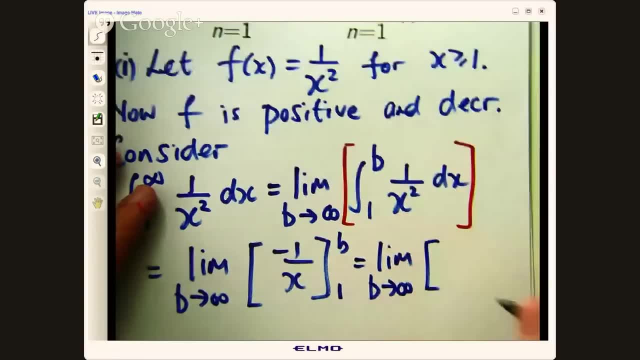 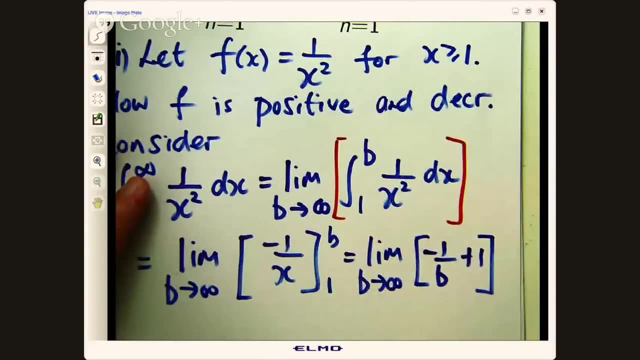 B to 1.. So let's put in x equals b and x equals 1.. So if I put in x equals b, I'll get that, And minus negative 1 gives us this. And now what happens to this? as b goes to positive infinity? 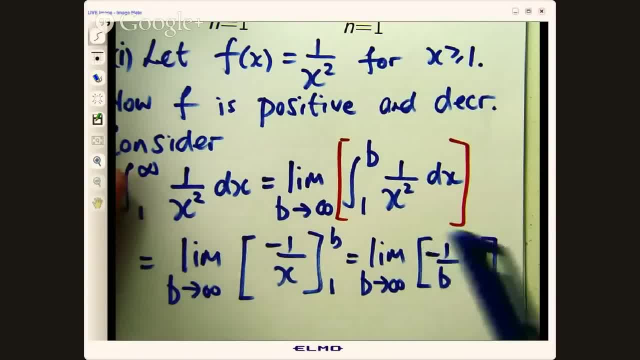 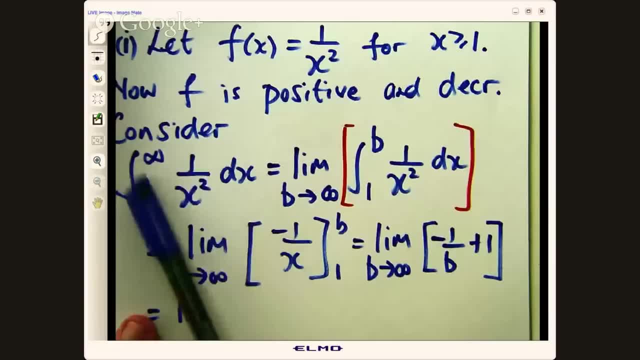 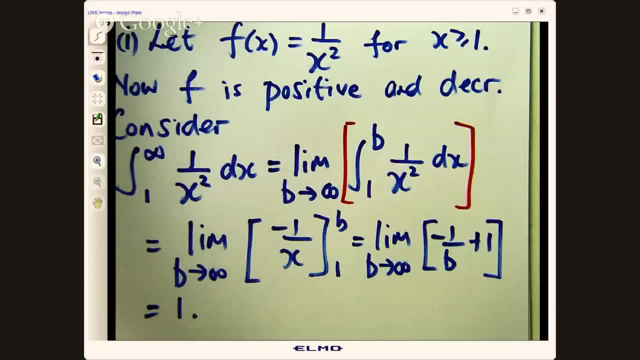 Well, this term will go to 0 and I'll be left with positive 1.. Okay so the important thing now is we know that the improper integral associated with our series converges to 1.. Okay so this integral test then tells us whatever the integral does, the original series will also do. 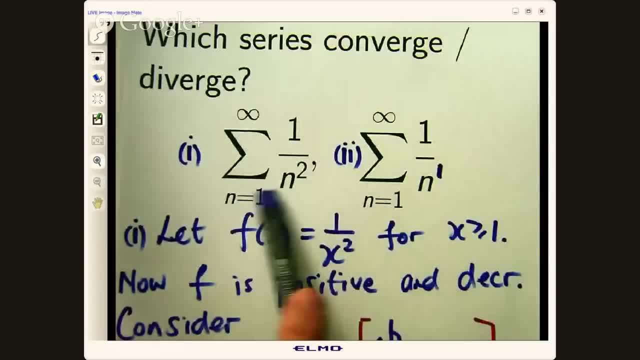 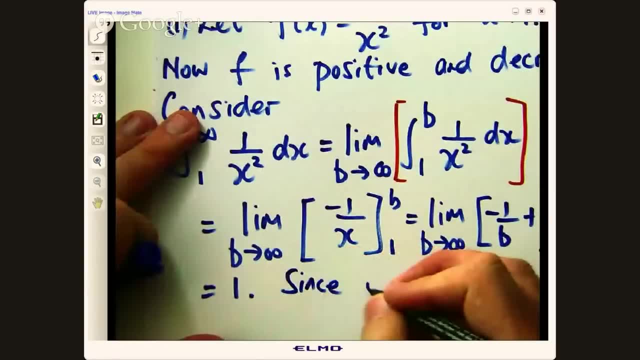 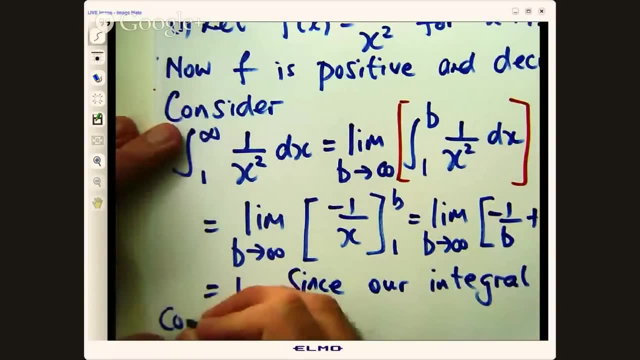 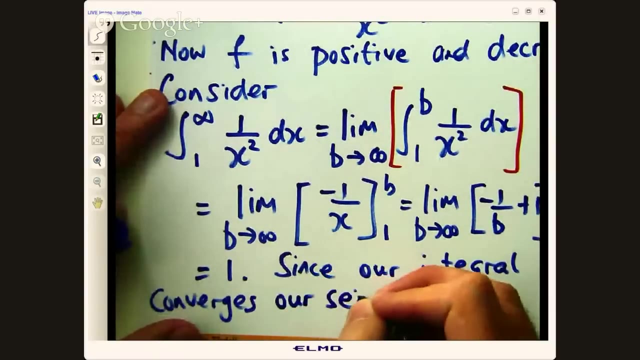 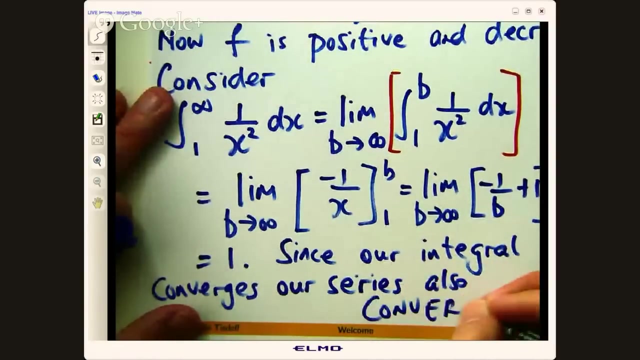 Okay, because this converges, this also converges, Okay. So let's write that down. Since our integral converges, our series- oops, series also- see if I can squish it in- converges Yes, Okay. so that is our conclusion. 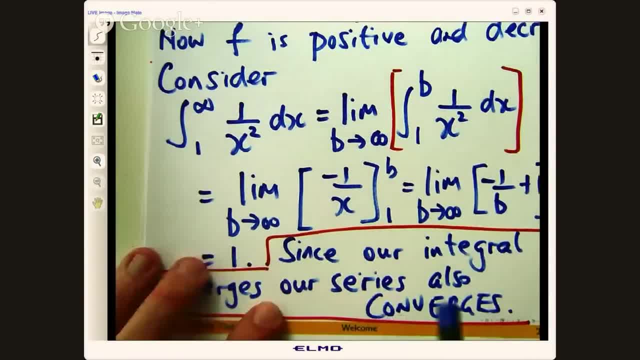 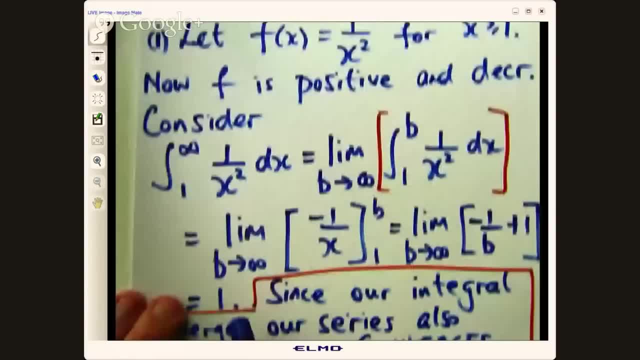 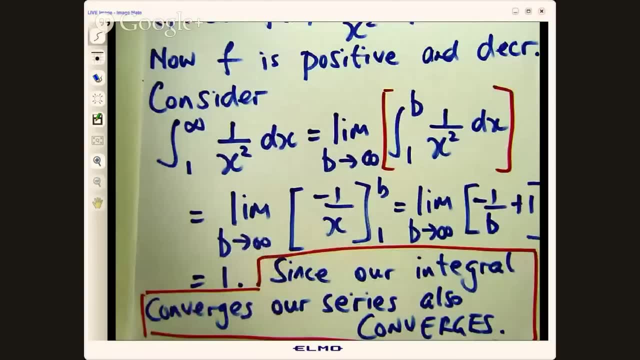 Now notice: we don't know what our series converges to. You might go: oh, it's got to be 1.. No, This series doesn't necessarily converge to this value here. All this tells you is that the integral converges and by this integral test the original series also converges. 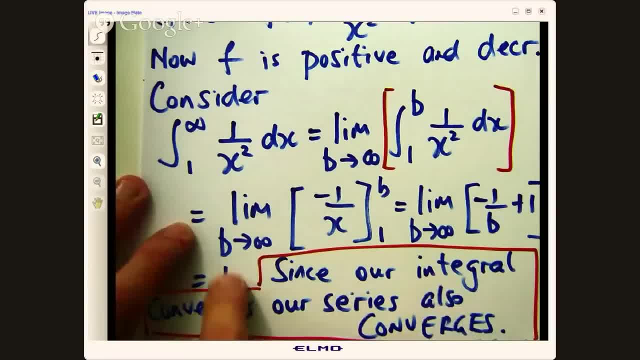 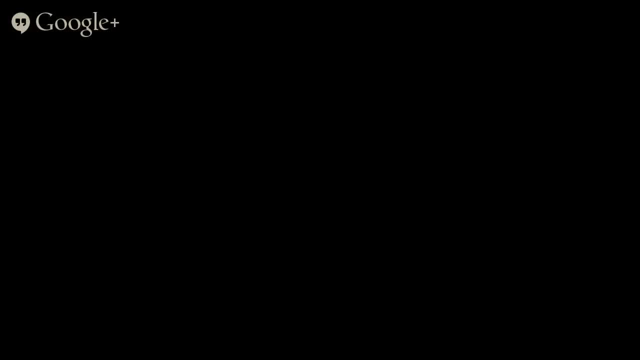 Basically, all it says is: the series converges. So this is the integral that converges to something that's less than or equal to 1.. Okay, All right, Let's have a look at part 2.. By the way, you might be asking yourself: why does this integral test work? 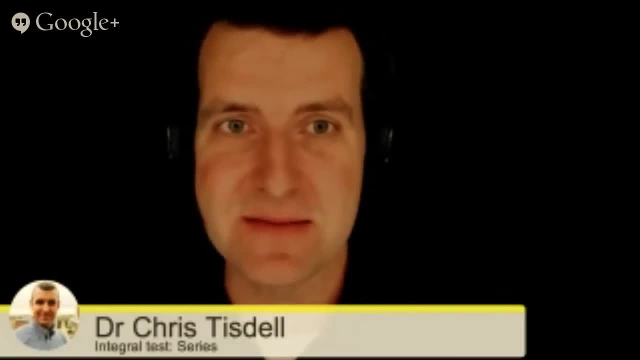 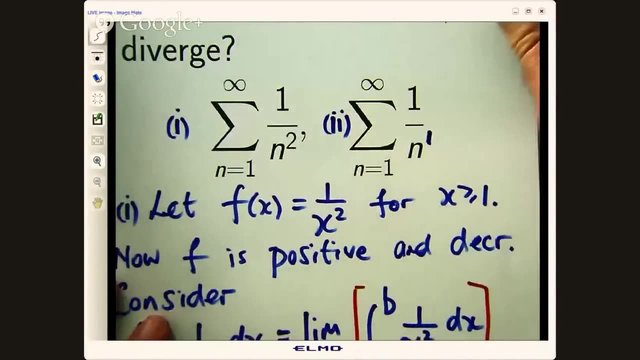 Well, I'll talk about that at the end, Okay, so let me show you another example. Let's do part 2.. 1 on n, the sum of that. Okay, so we're going to run a similar line of argument here. 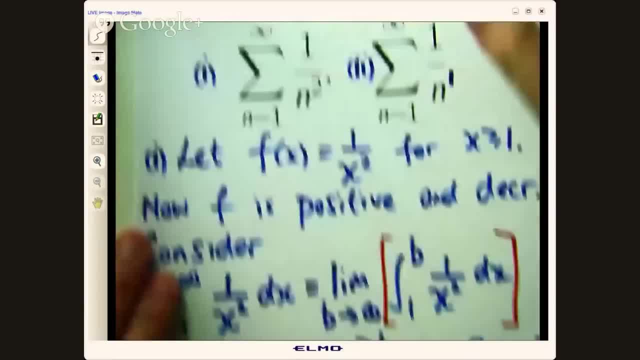 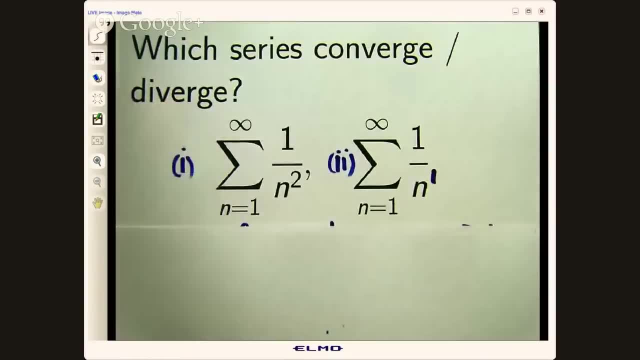 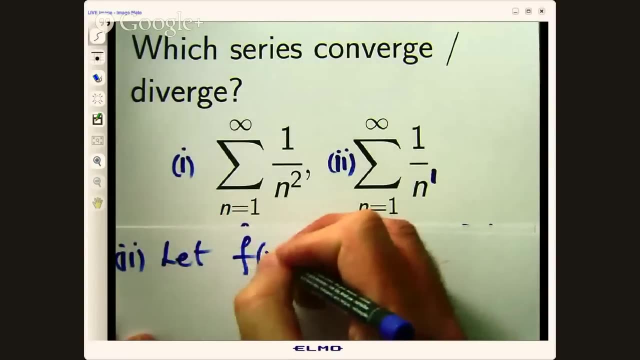 So f of x will be 1 on x for this one. Okay, So let's start a new page. So for part two, let f of x be 1 on x for x greater than or equal to 1.. All right, and similar to the two conditions. 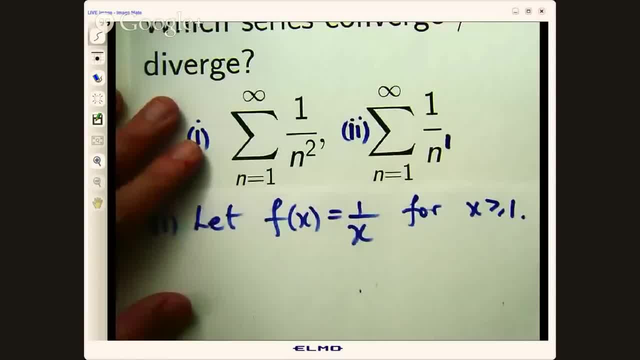 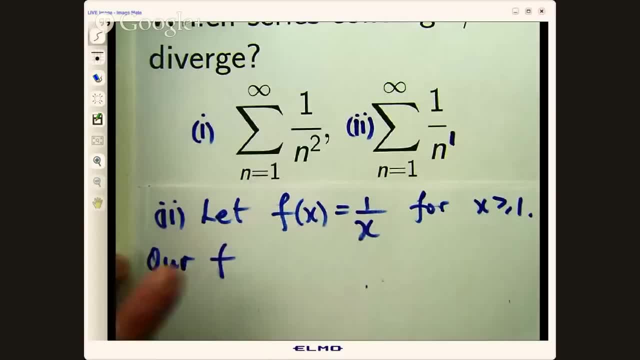 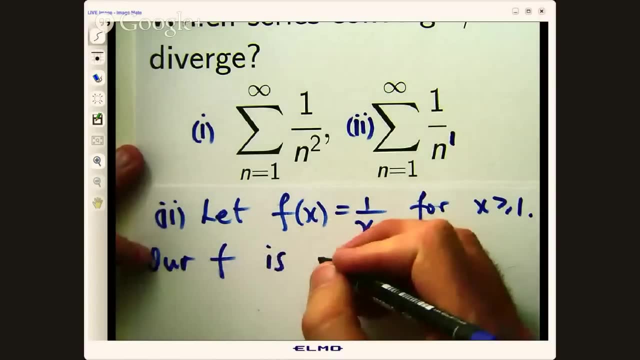 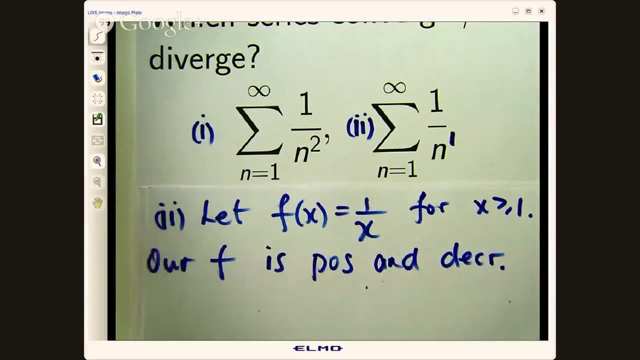 that we had over here- f- positive and decreasing- is also true for this function here. If those two conditions aren't satisfied, then you can't use the integral test. So our f is positive and decreasing. Okay, so just positive and decreasing. 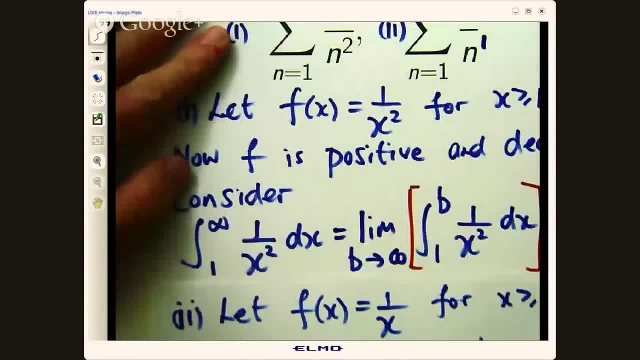 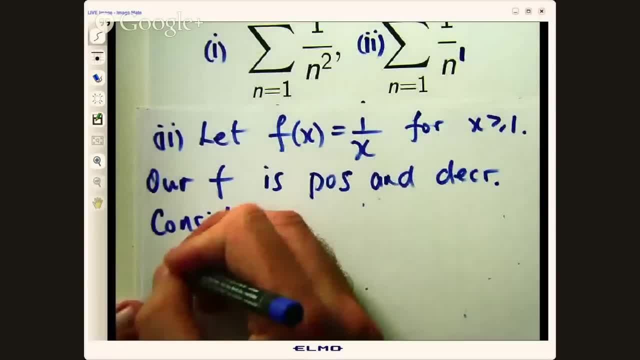 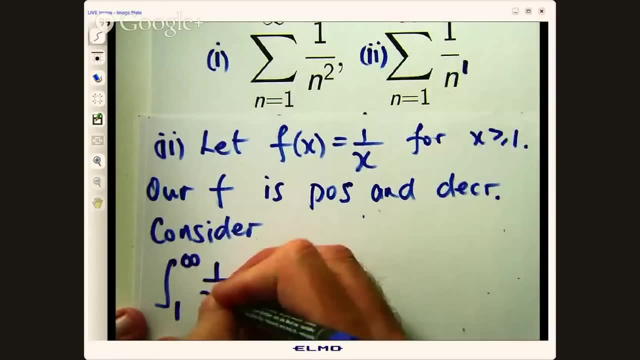 All right, so let's consider this improper integral now. Okay, So we'll be integrating from x equals 1 up to positive infinity of 1 on x dx. Okay, so let's just repeat the steps that we did last time. Let's write this as a limit. 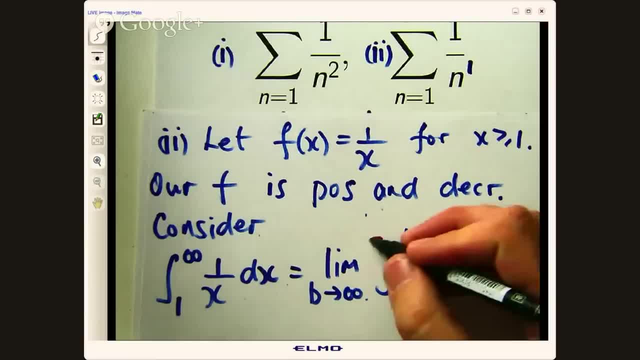 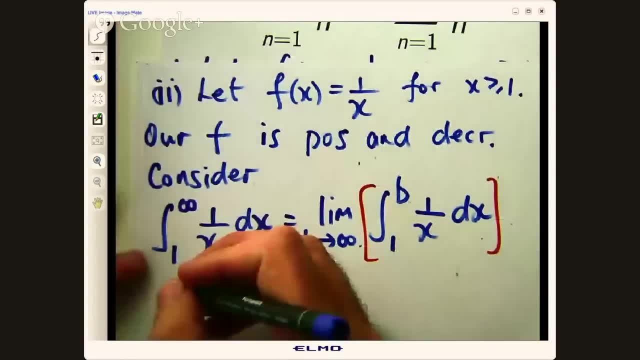 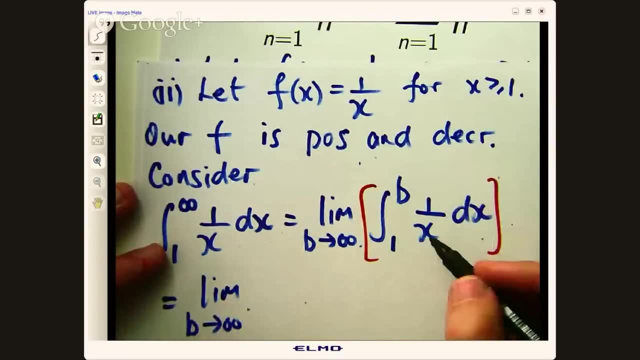 Okay, and we will work out the integral first and then we'll take the limit and see if it converges or diverges. Okay, All right, so we integrate this. x is positive, so it's going to be a logarithm function. 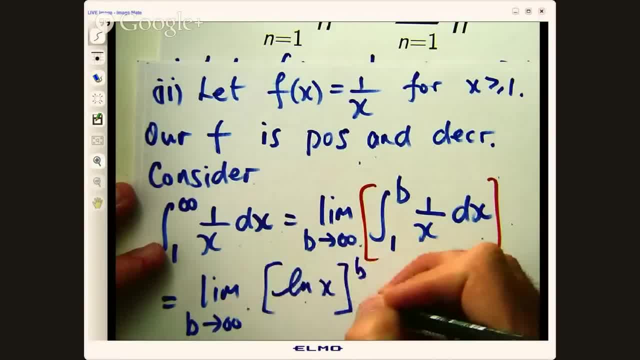 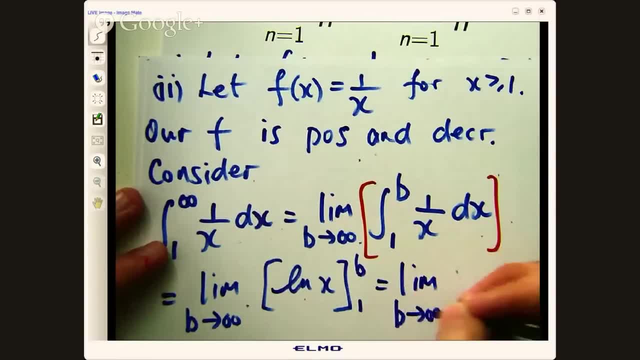 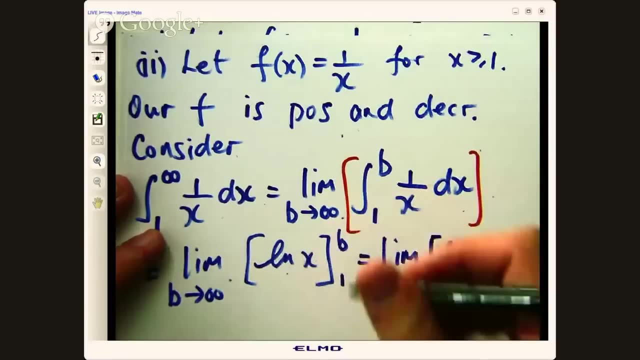 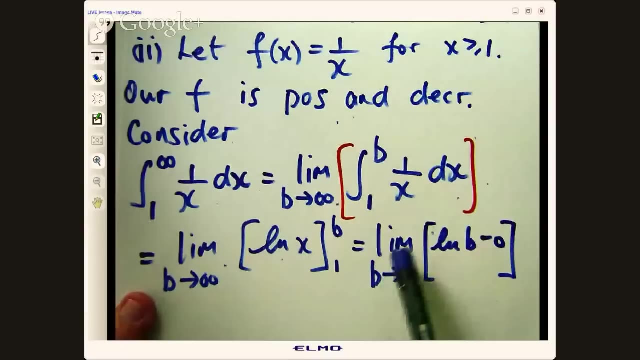 natural logarithm function And if I plug in, what have I got? I've got log of b minus log of 1.. So log of 1 is 0. So basically I'm just taking the limit of the logarithm of b, as b goes to positive infinity. 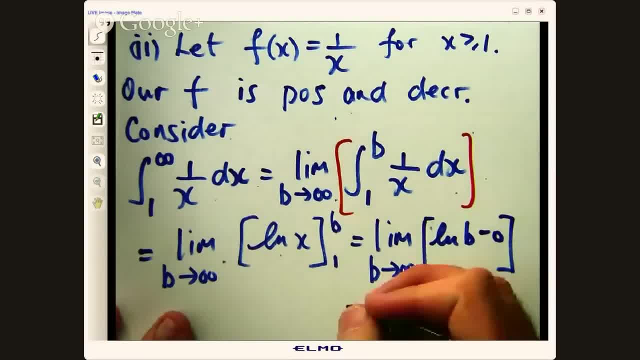 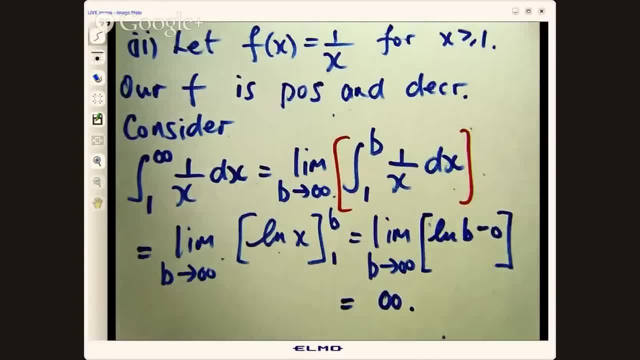 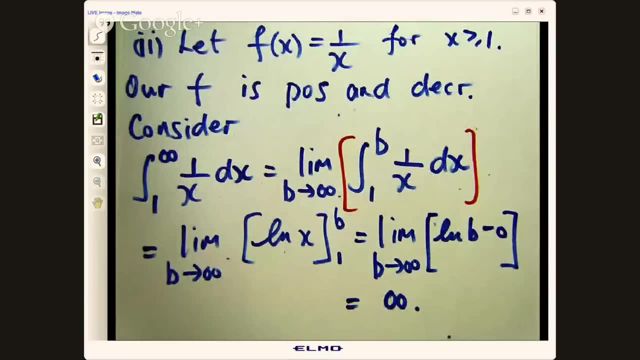 Now the logarithm function is an increasing function, so this diverges to positive infinity. Okay, so in the previous case it was a finite number, it converged, But here it goes off to positive infinity. So let's use the same idea. 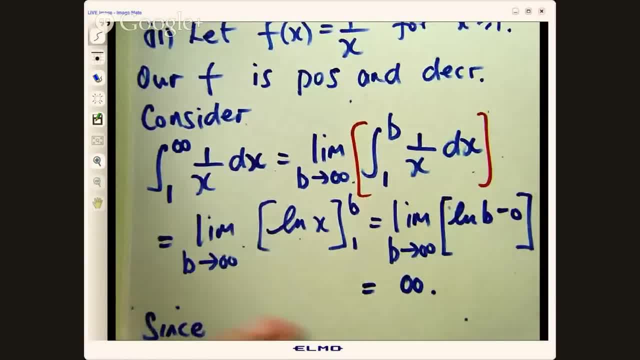 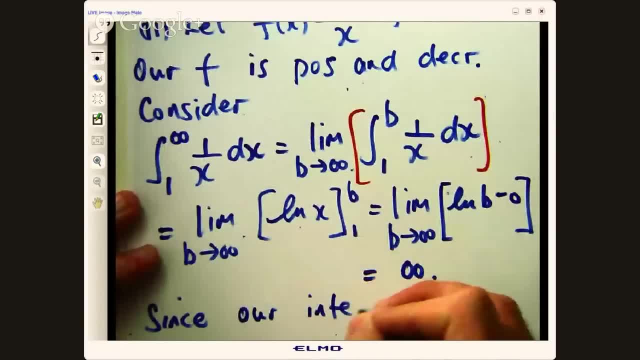 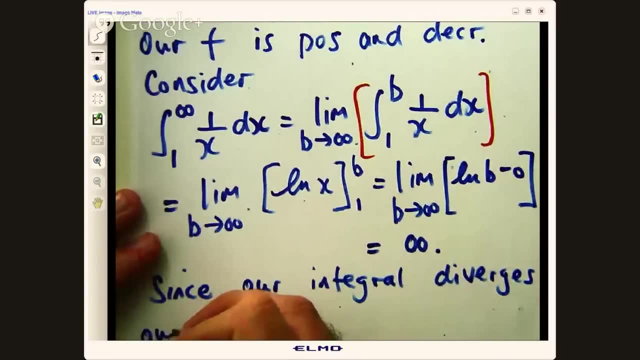 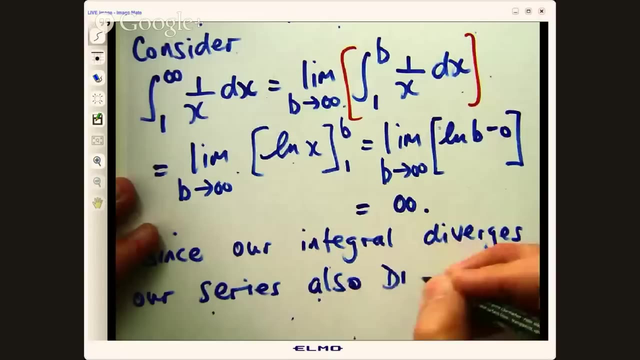 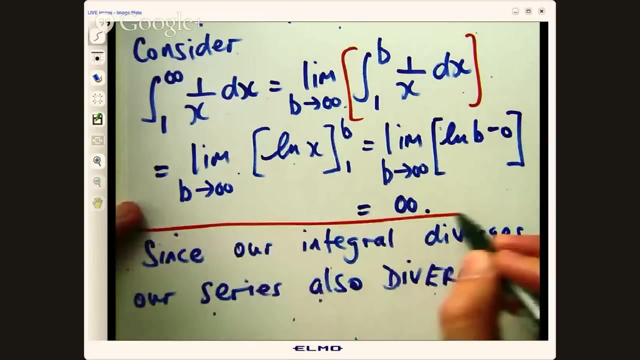 Whatever the integral does, the original series must also have that behavior. Okay, so let's make a conclusion then: Since our integral diverges to positive infinity, our series must also diverge. Okay, so this is our conclusion for the second series that we were given. 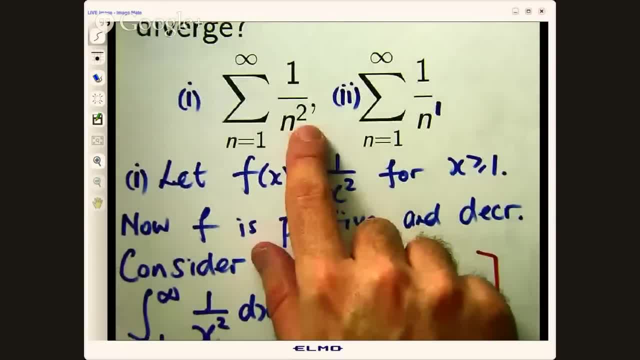 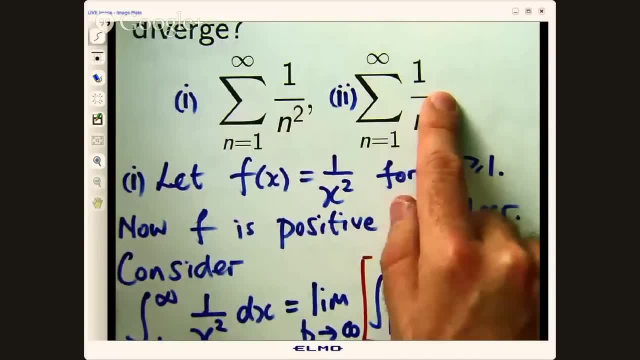 Okay, So you can see we haven't really changed much here. The power is just: it's a 2 here and it's a 1 here. This converges and this diverges. Doesn't seem to be much difference there, Okay. 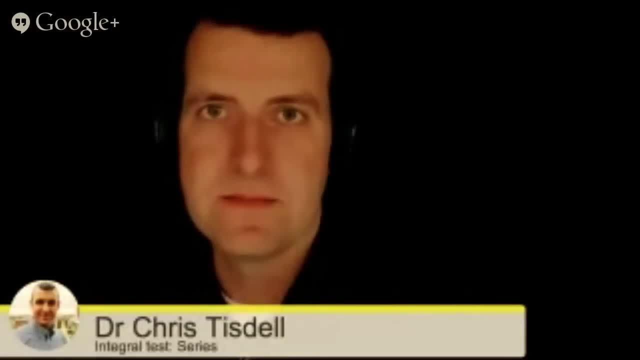 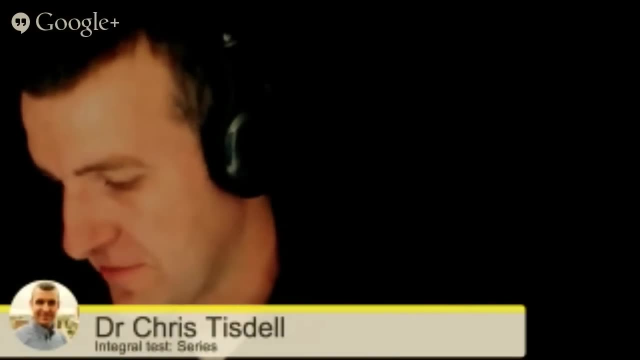 But I've got a full function, but it's a 2 here And the function here is positive infinity. So that's just a two which will go by two. We don't need any other function here, But we need to use this to make that difference. 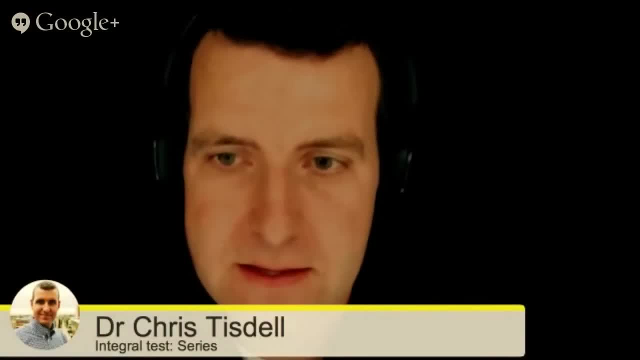 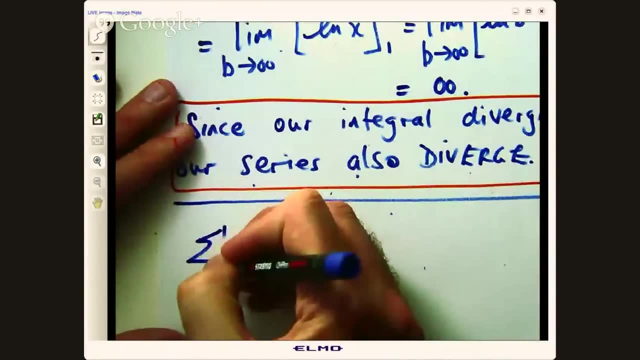 So it's a 2 here, So that makes it a 3.. If it's a 2, it's a perfect integral. Is there a general rule for these p-series? Yes, there is, and I'm glad you asked. Let me write it down for you.